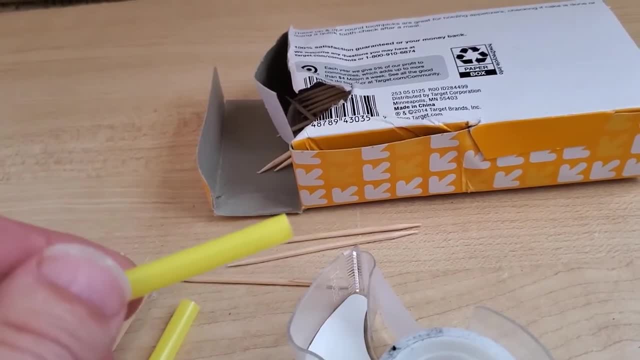 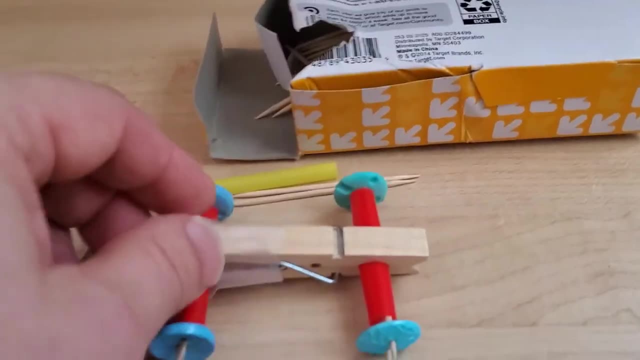 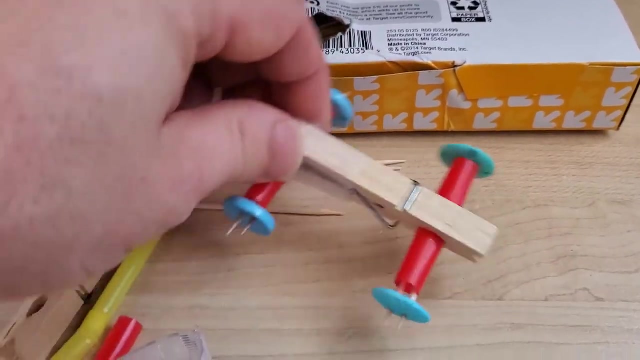 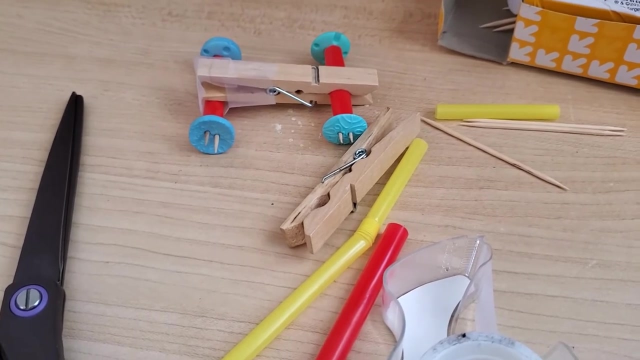 straw that I was planning to, because this is too small for both of the toothpicks to fit inside and for the wheel and axle to still roll. So this is my design for my very own clip car: clothespin- my clothespin car. It took me a little while to remember the name. 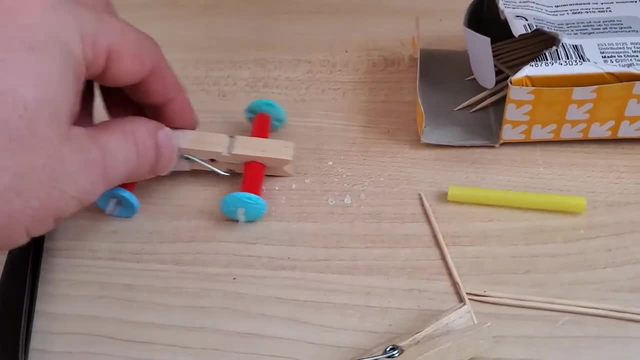 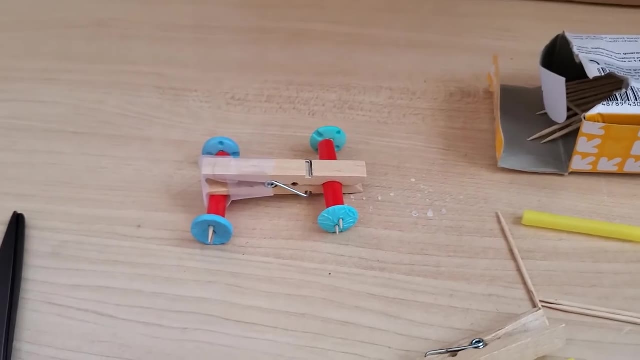 And so this, This will work quite well for making the car. I'm going to go over the steps in just a little bit and I'll go ahead and show you how I make mine, And after that you can do some experiments to. 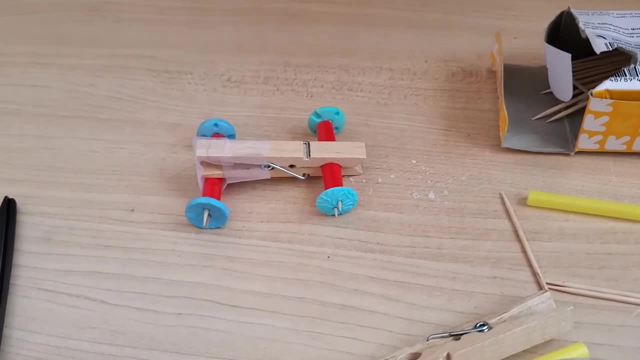 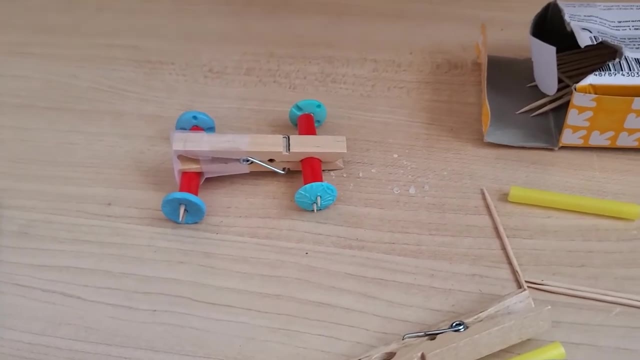 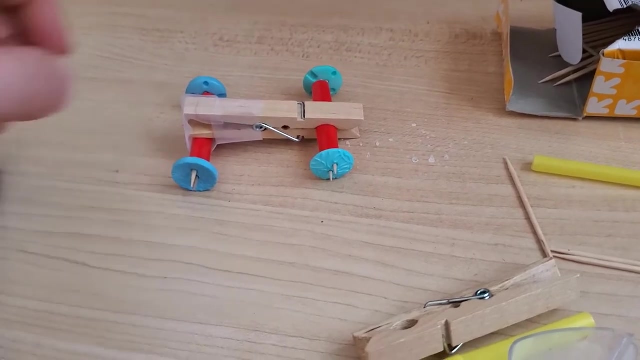 see how well yours rolls. Now, if yours doesn't roll all that well, I'd like for you to become an engineer. put that engineering cap on and think about how you can change it to make it even better. For mine, I would probably add maybe a little bit of hot glue in order to make it work. just a little. 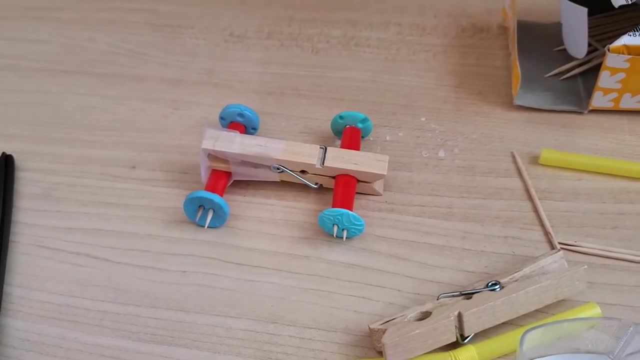 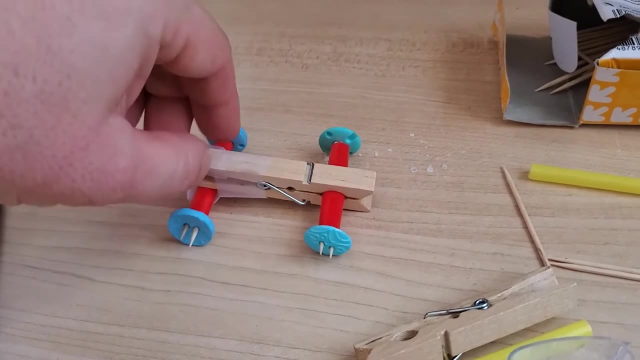 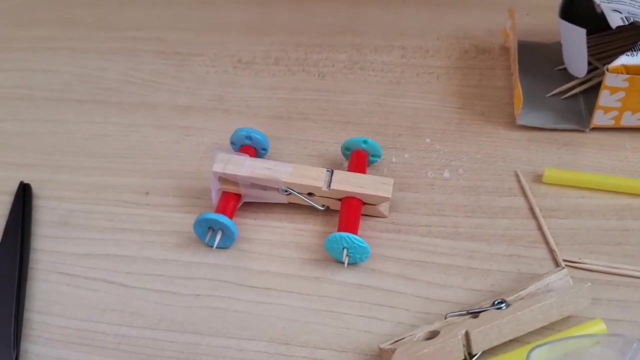 bit better, roll a little bit straighter, and I might make a few more changes Today. our question for the day is: how will a car roll in on different surfaces? And I want you to think about what might be stopping a car from rolling on different surfaces or if it rolls further on. 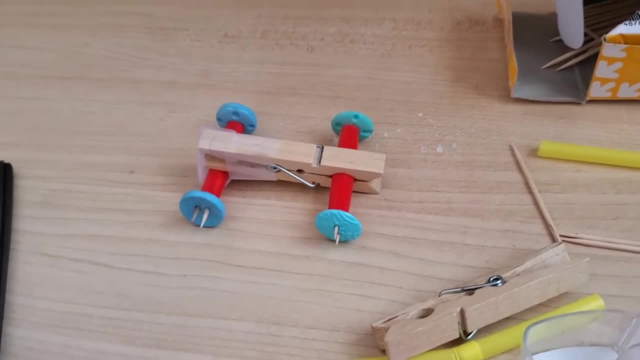 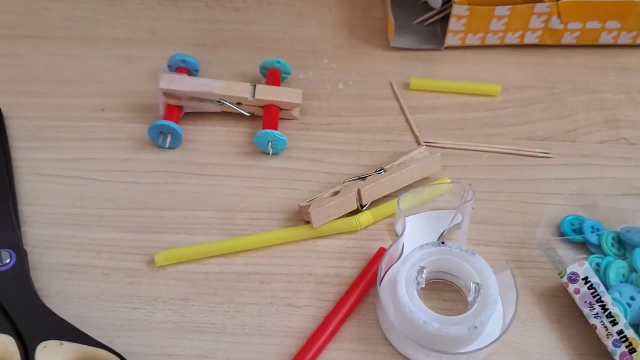 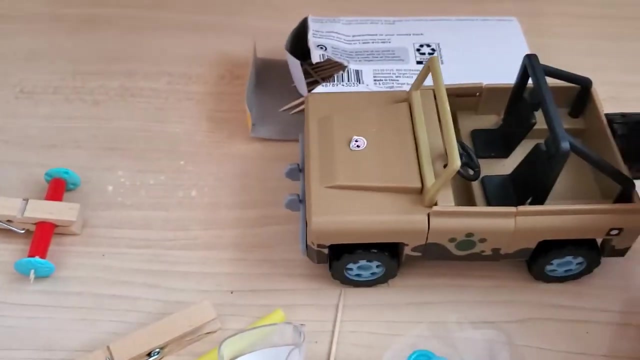 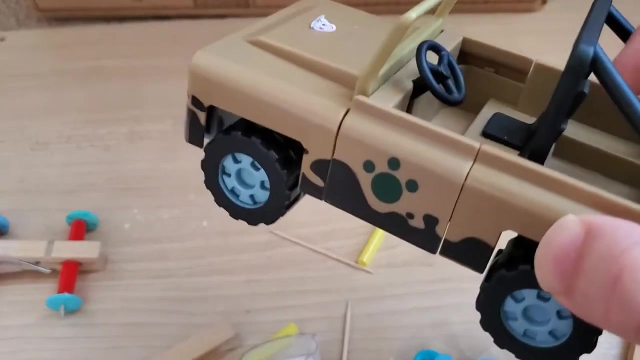 one surface And then I'll stick you up to speed so you can see how it rolls on each surface. But before we go there, I have gotten some wheels and axles right here, and here is one wheel and axle. I think this is a toy car. I'm going to go ahead and put this wheel. 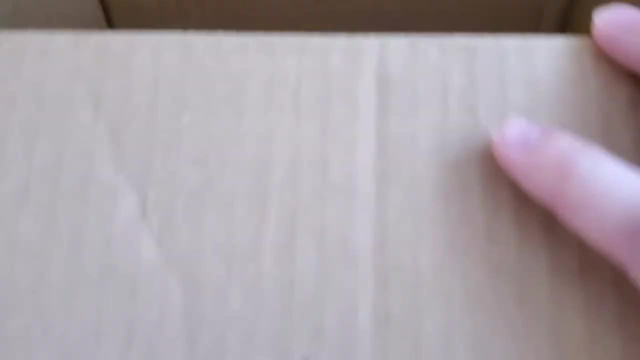 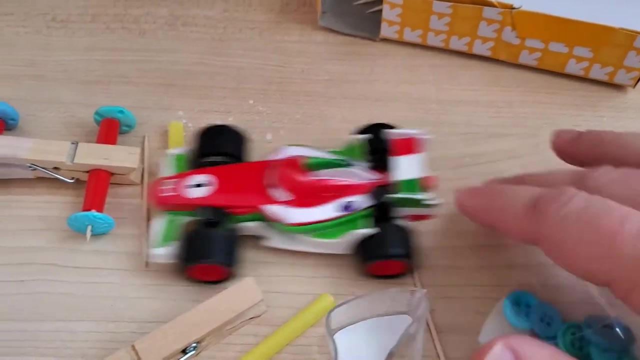 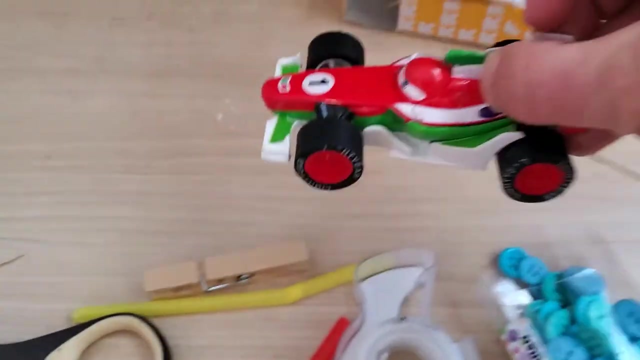 and axle inside my simple machine box. so it's going inside there and I found two others. This is a little sports car and it actually rolls quite well. I think it has a little motor you can pull to have that roll. That's going. 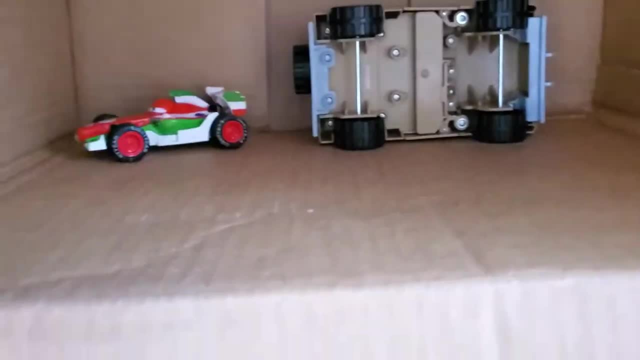 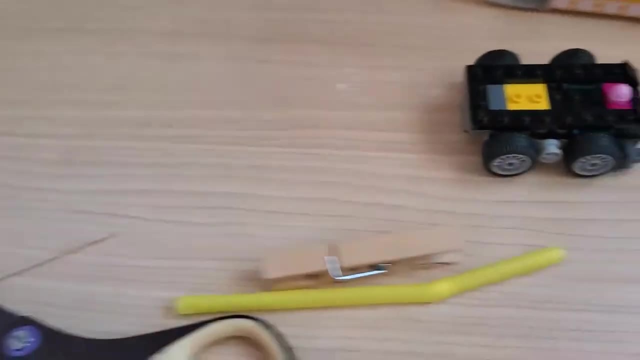 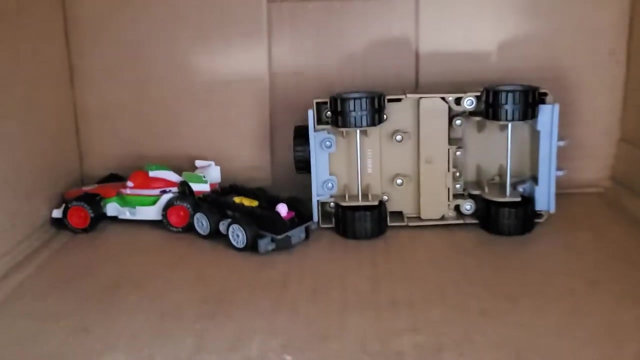 to be a lot of fun during this unit, So I'm going to drop that. It's going sideways in as well, And we have a half-built Lego car with the wheels and the axles on this side, So I will drop that into here as well As we go through learning about the simple machines. 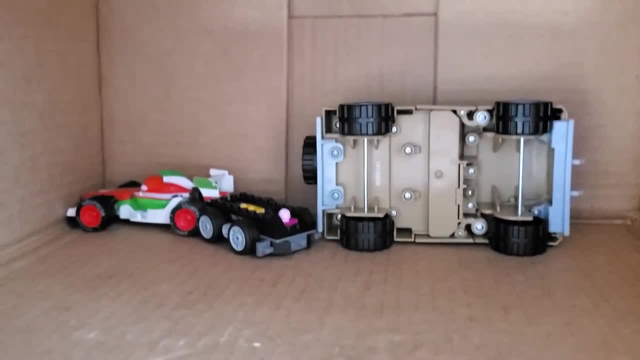 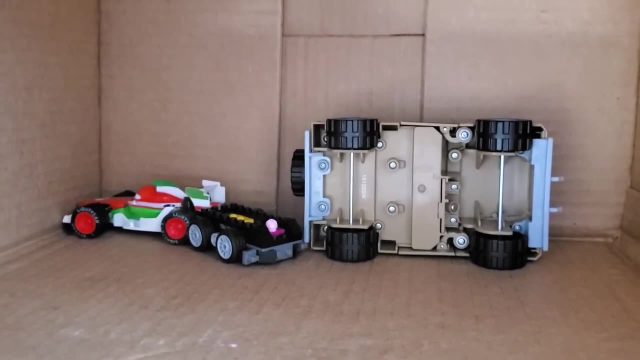 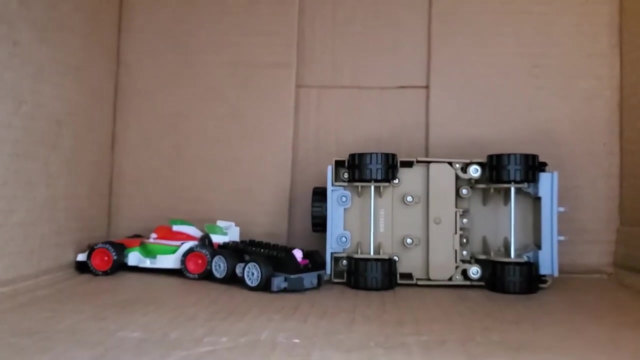 this week we're going to be adding more simple machines into this car and in the following week it will be very useful for us. So keep on putting your simple machines inside. and all the boxes are looking great. All the boxes are looking great, So we're going to go ahead and switch to a video. 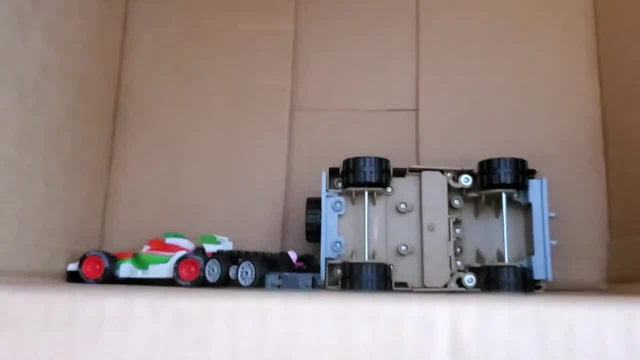 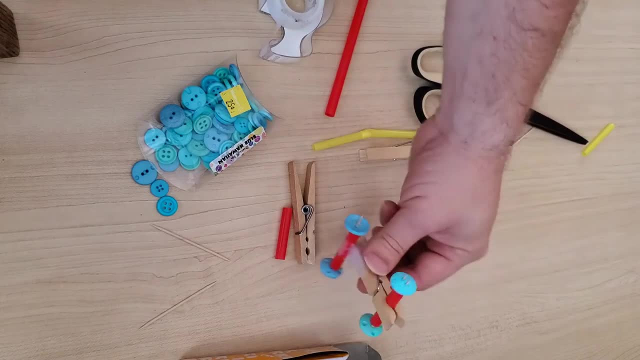 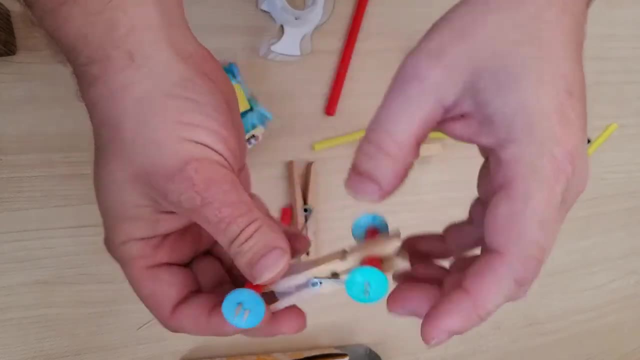 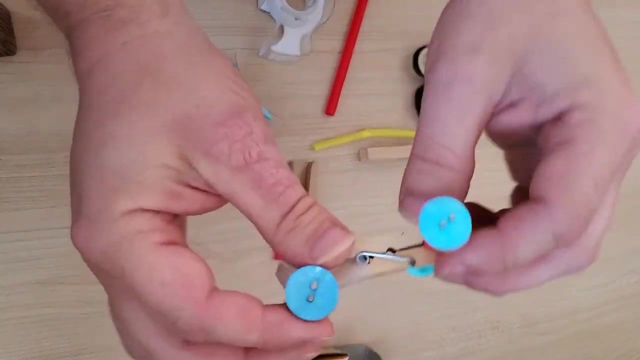 To assemble the car, you will need a few different items. You can see that we will need four different buttons that should be the same size for each set of wheels. For this we would need four toothpicks as well, one paper clip, some tape to adhere it to. 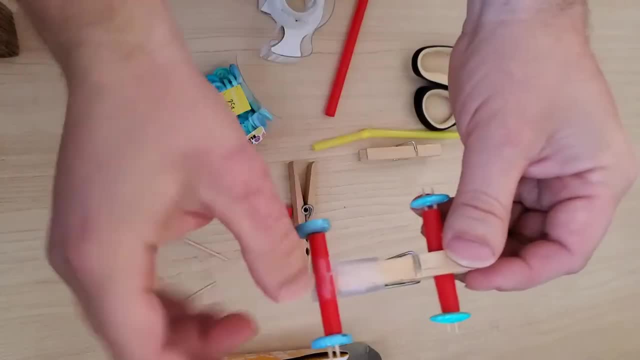 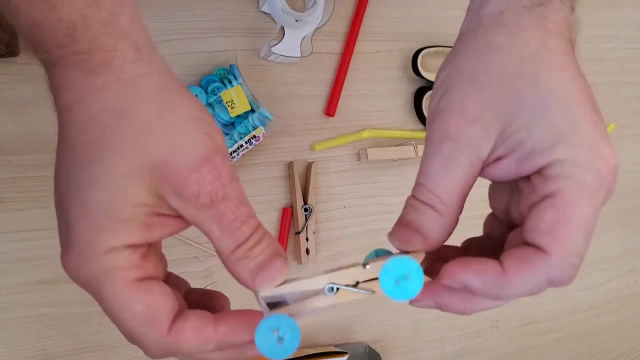 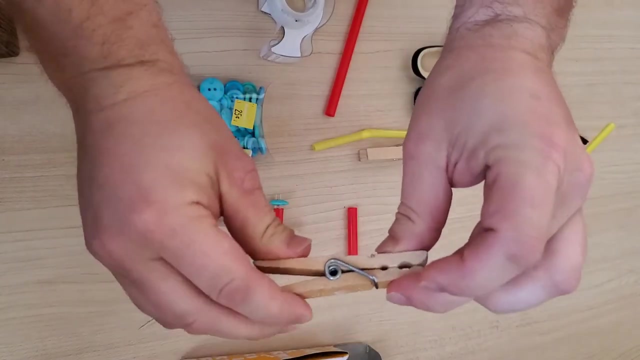 If I had a little bit of hot glue that I put on, then that might make it last a little bit longer, make it a bit more secure. So that's something that you can think about. Now. I had a different size of closed pin and I wanted to see if the different closed pin 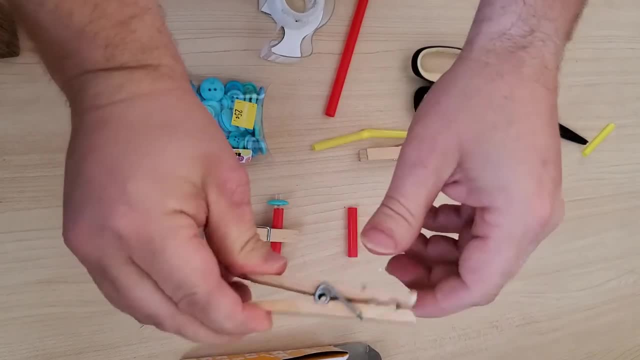 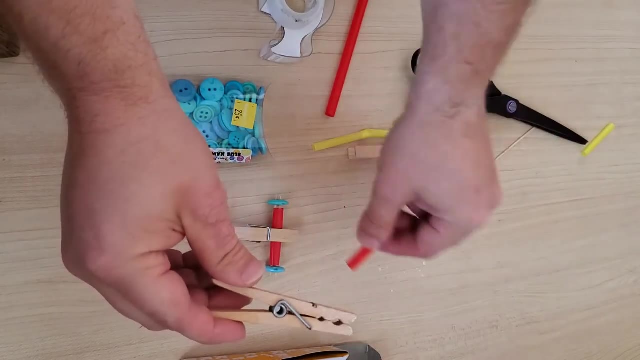 might have a different reaction. This one is a lot, quite a bit stronger, so as it pinches, it's going to pinch a lot firmer, which wouldn't be very good for the straw, because it doesn't have that much thickness. So I'm going to, when I put this in, also put a little bit of tape on it. 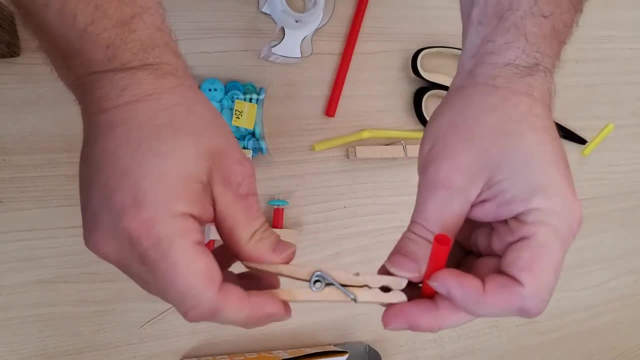 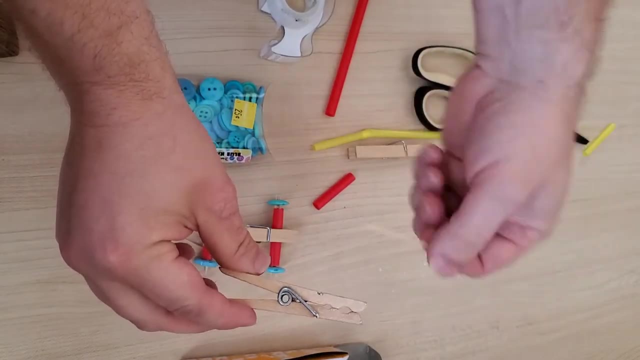 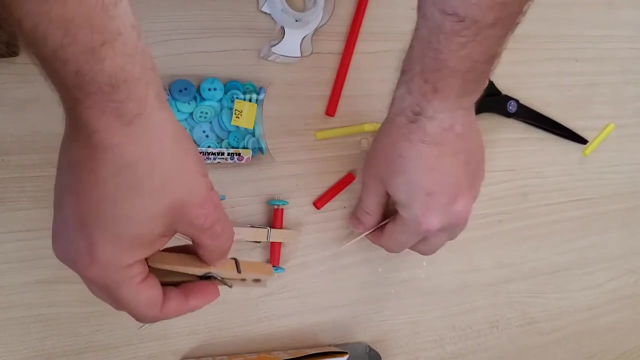 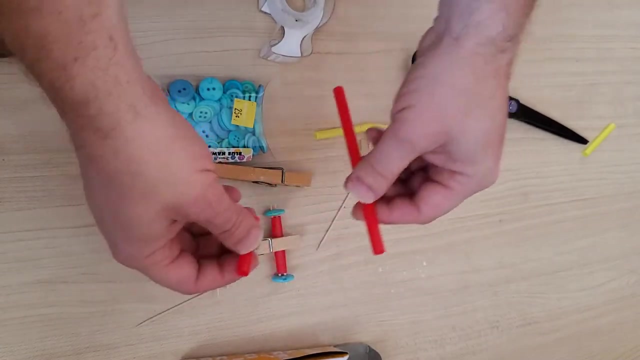 So that the force with which this closed pin closes doesn't stop the toothpicks from spinning around which the toothpicks are the axle. so if the axle can't spin around, then the wheel and axle doesn't work. Okay, so this is the thickness that I had for my closed pins and or for the tubes that 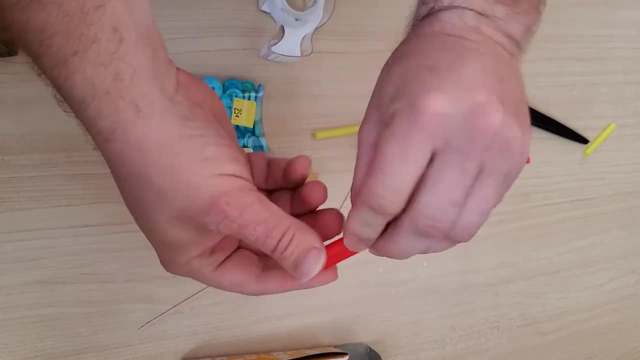 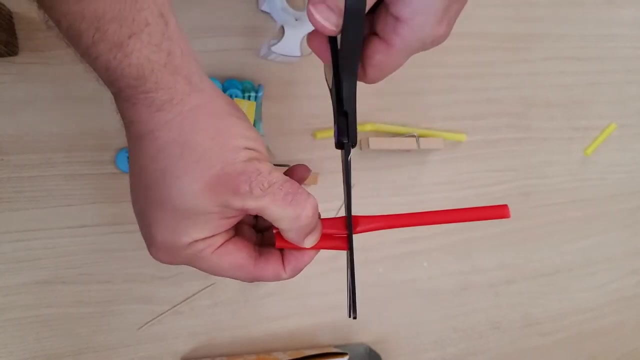 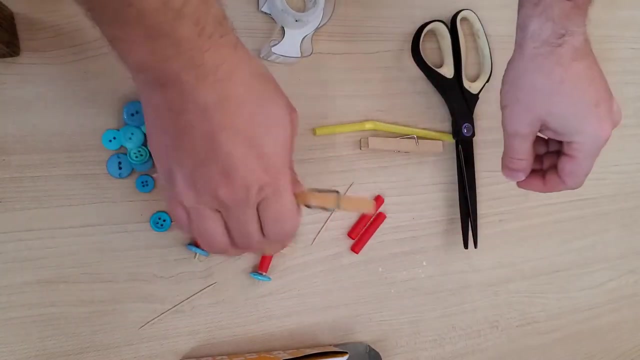 the wheel and axle goes through. So I'm going to put a little bit of tape around the sides so that they don't go through. So I'm going to just try to make it about the same And just eyeball it right about here And the straw goes flying. Okay, so we're ready to go ahead and put a little bit of 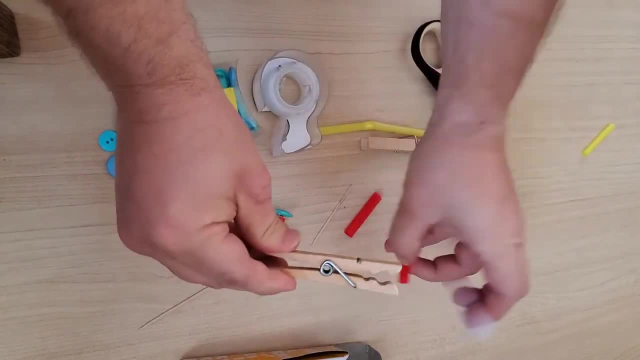 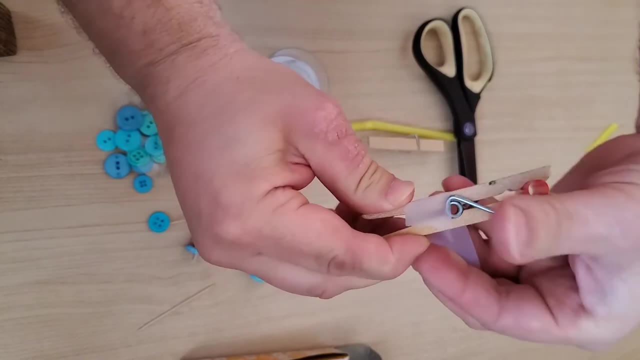 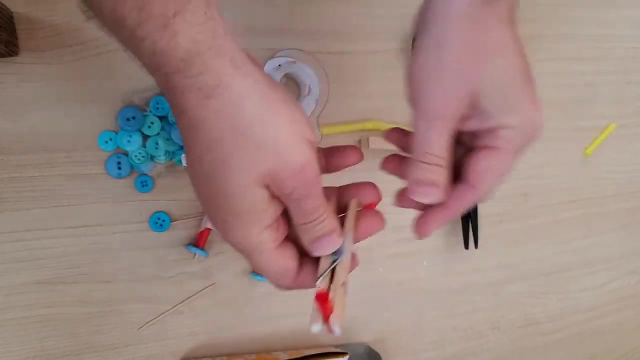 tape on it, And if I use stronger tape then it would be a little bit stronger. but that's okay. I just want to make sure it holds for a little bit Little experiment. I'm not going to be racing it with anyone. There we go. Okay, that seems to be. 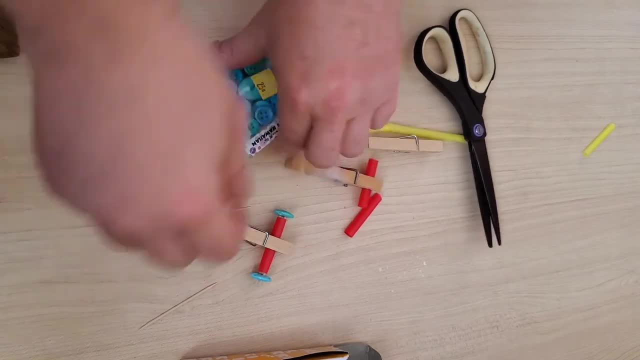 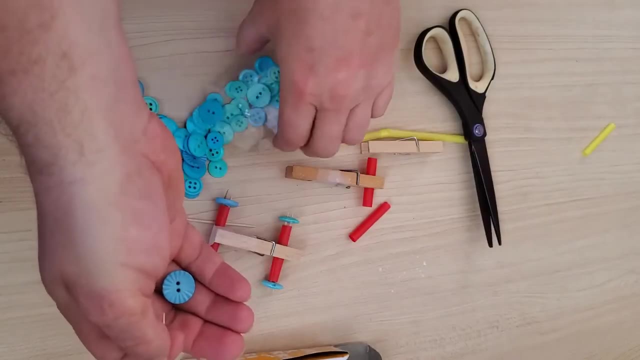 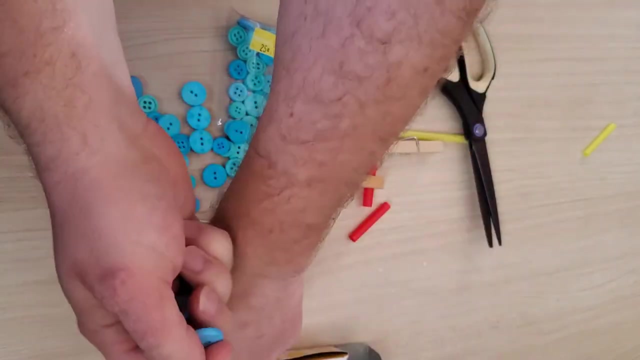 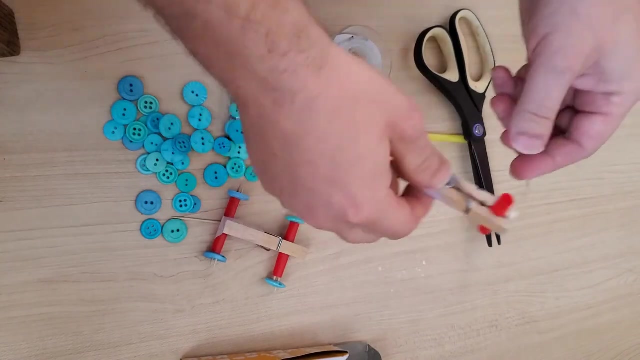 holding. well, So I need to take two buttons that are the same And let's make it look really snazzy and make sure that they're exactly the same buttons. Okay, here is one, And these two together are my axle, Which I will slip through here, And that doesn't look like it's crimping. I'll put it right in through. 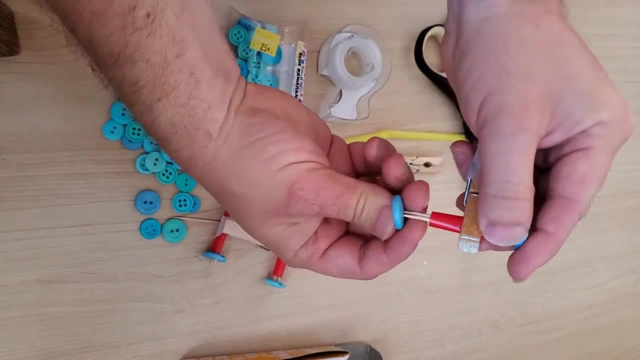 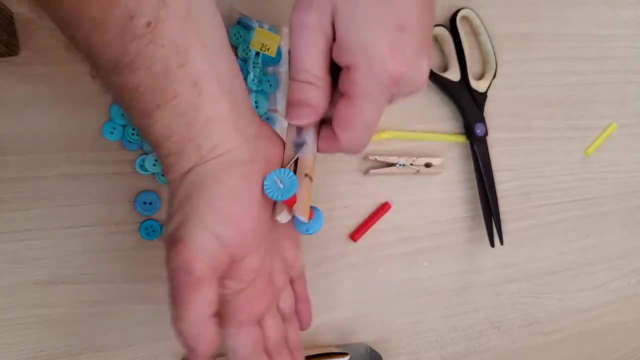 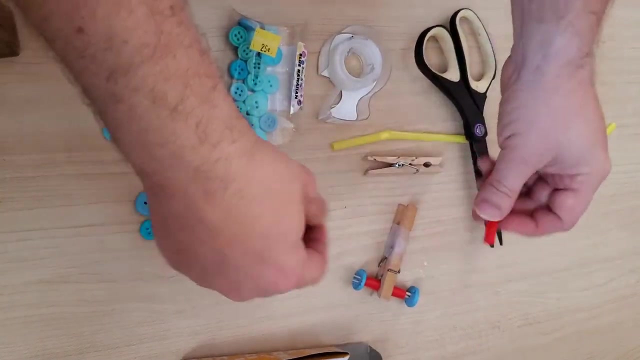 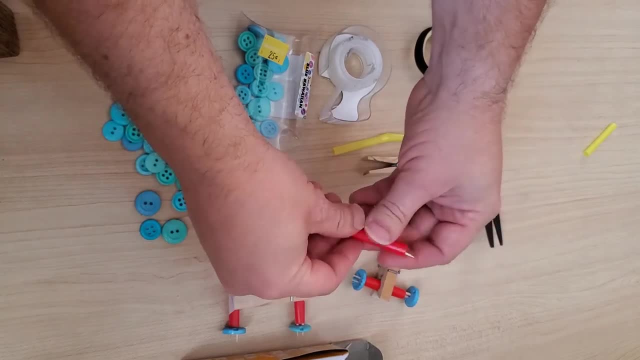 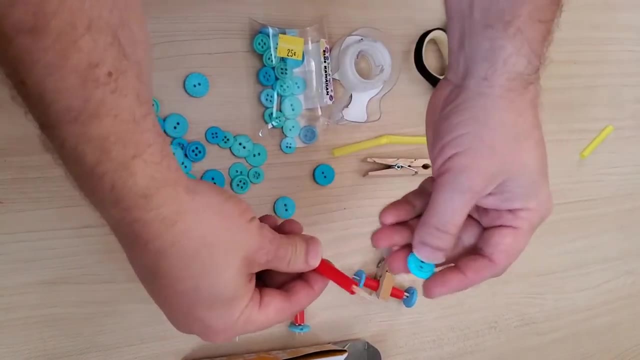 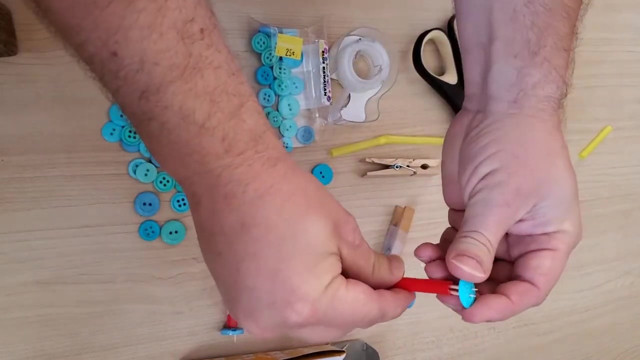 I need to get two toothpicks, Slip it through And then put two wheels on, And those don't quite match. So let's see if we can find some that do. Look, here we go. Nice, we've got the same pattern. 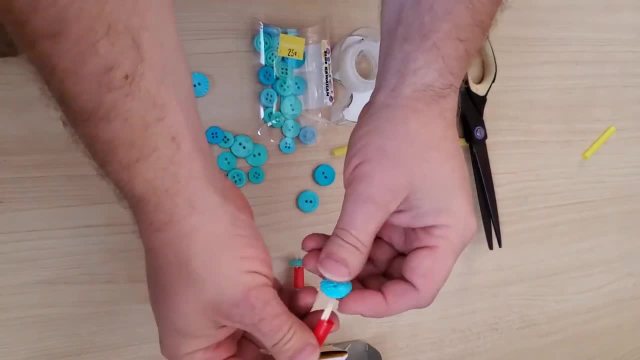 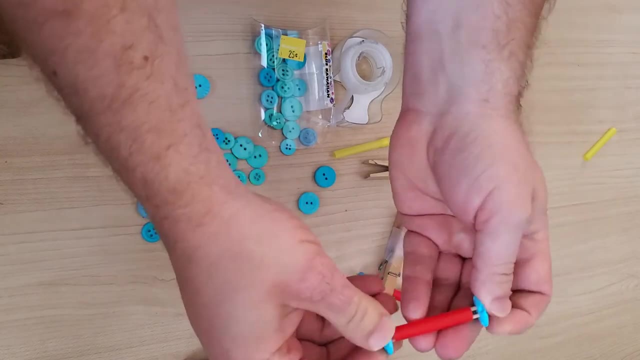 That's okay. If you want yours to be different, if you want yours to look some other way, go ahead and make it how you want it to be. If you want to paint your wheel by hand, you can do that toothpicks. if you want to paint your clothespin. if you want to use 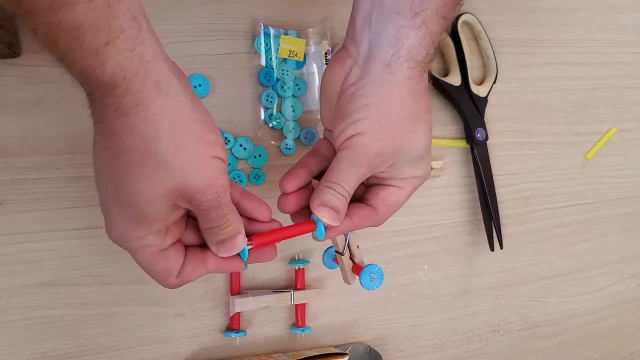 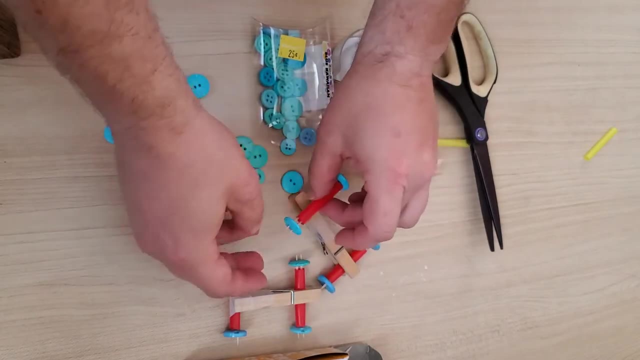 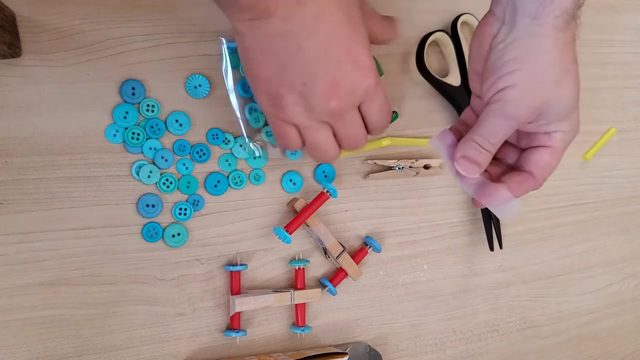 different colored tape. if you have it, please do so. Make this your own work of art. Okay, now I'm ready to tape the wheel and axle onto the back and I can test it and it's spinning quite well. I'm just going to get a little bit of tape and tape it.